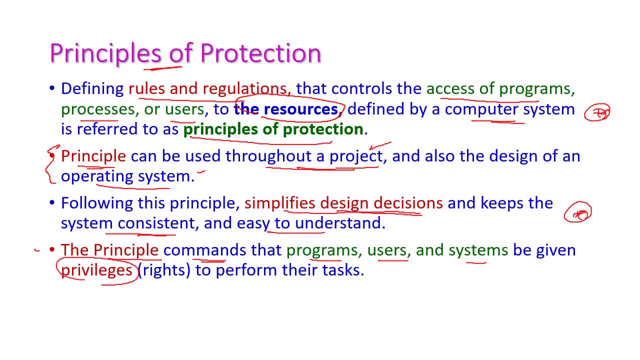 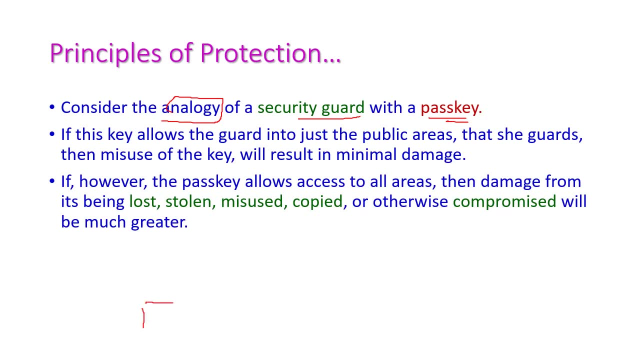 And be given the privileges to perform the task- That is the principle- will provide rights to perform their task. Let us see one analogy. that is a security guard with passkey. That is, we are having many areas, for all the areas, A security guard is there. Okay, the security guard is having one passkey. 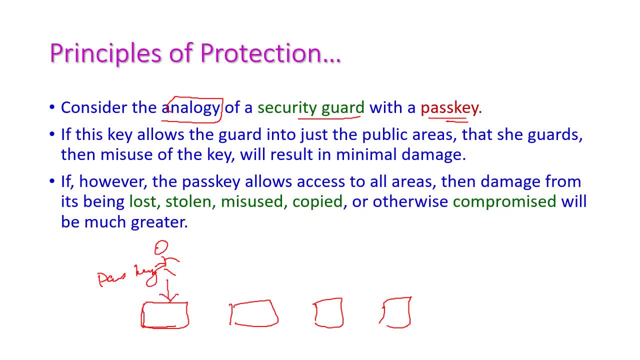 One passkey. This particular security guard is having one passkey. The security guard is going to guard this particular area, right? Suppose, if the passkey is misused, then only this particular area will be affected. That is, damage is very minimal. 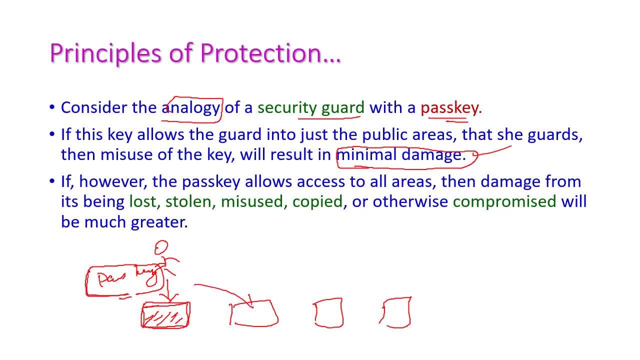 Suppose, if the same passkey is used for all the other areas, that is, misused for all the other areas, then what will happen- That is, lost, stolen, misused, copied or otherwise compromised- will be much greater. Hence the designing of principles of protection is very, very important. 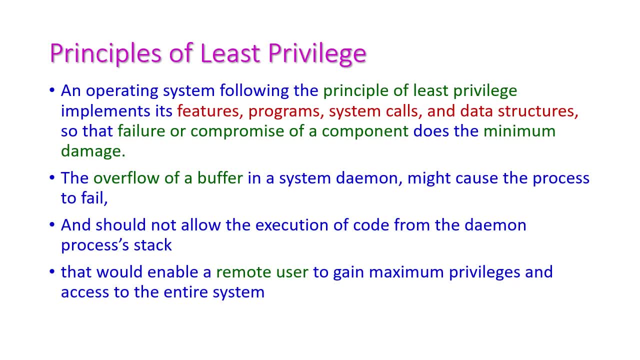 When come to designing an operating system, it should follow the principles of least privilege, which implements its features, programs, operating systems, that is, system calls and data structures, so that the failure or compromise of components does the minimum damage. So we have to implement. 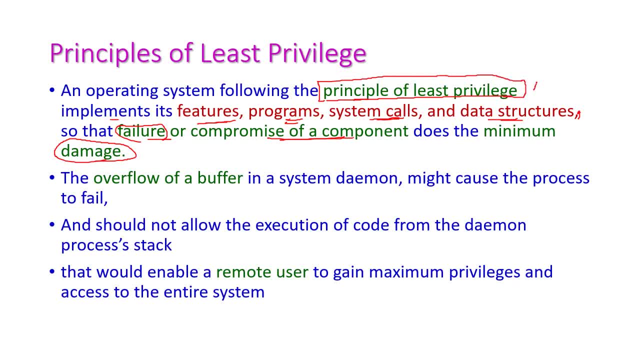 Or we have to follow the principle of least privilege, Isn't it So? if it is least, then the damage will also be minimum. Here, the overflow of a buffer in the system demand that might cause the process to fail, And we should not allow. 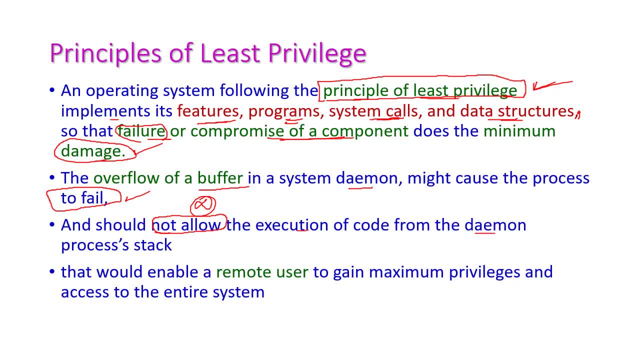 Okay, we should not allow the execution of code from the demand process stack. What will happen? Otherwise? it will enable the removal. So we need to protect our system from the remote user to gain maximum privilege and access the entire system. So we need to protect our system from the remote user to access the entire system. that will cause a very big damage. 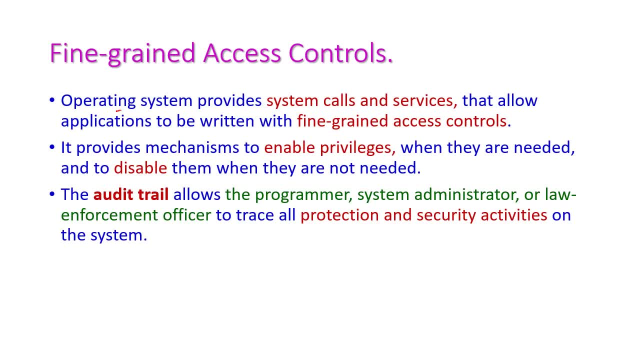 And next let us see the fine grind access control. Here the operating system provide the system calls and services. We have already seen the system calls and services of operating system which allows application to be written in. That is fine grind access control. 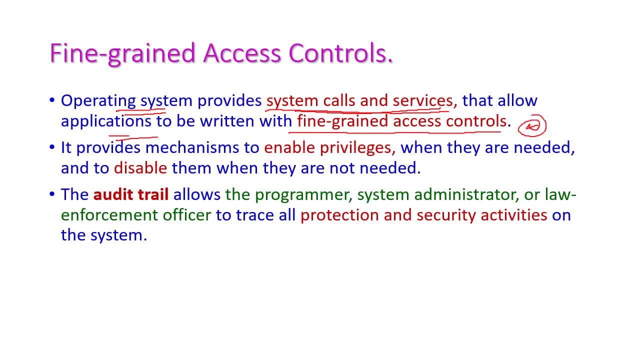 And this particular technology provides to enable the privilege when the users are needed or disable the privileges when they are not needed. Okay, for this purpose, the fine grind, access control is important, And the next one is the audit trial, which allows the programmer, the system administrator or law enforcement officer to trace all protection. 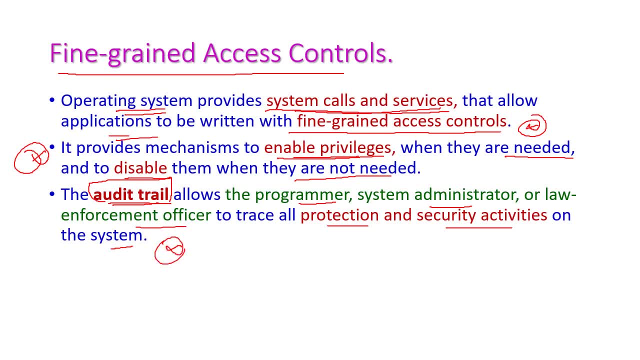 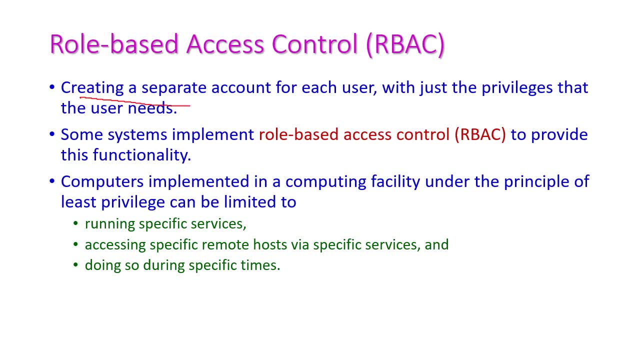 and security activities on the system. role-based access control, that is, creating a separate account for each user with just privileges that the user needs. so, based on the user's requirement, we can give access to all the users and some system implements the role-based access control to. 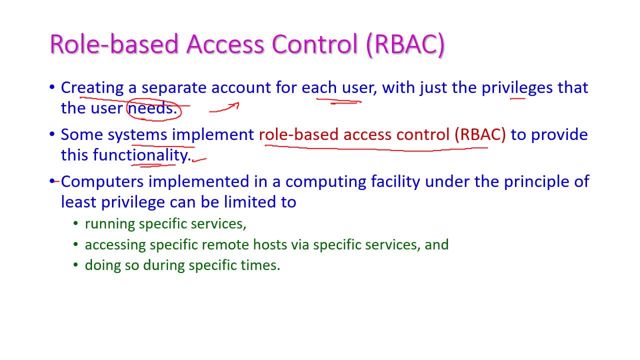 provide this functionality. okay, that is, computers implemented in computing facility under the principle of least privilege that can be limited to running a specific services that is a particular user should run. are you used to access only a specific services and accessing specific remote host via specific services and doing so? that is, doing all these things during the specific 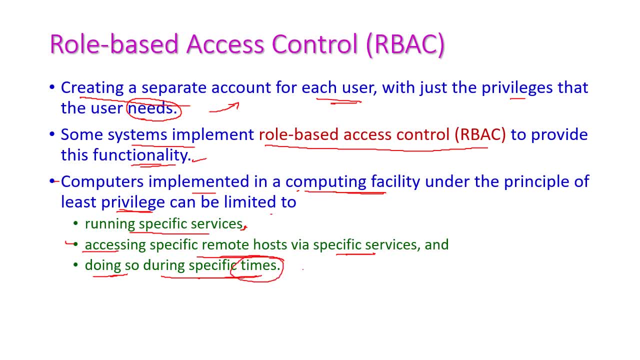 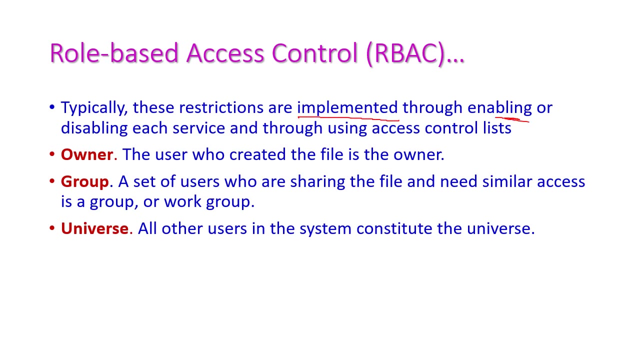 time, that is, which user can access which particular resource at what time and by using which particular resources. okay, that is, which particular system. all these things should be defined by using this role-based access control. these restrictions are implemented through enabling or disabling each services and through using the access control list. 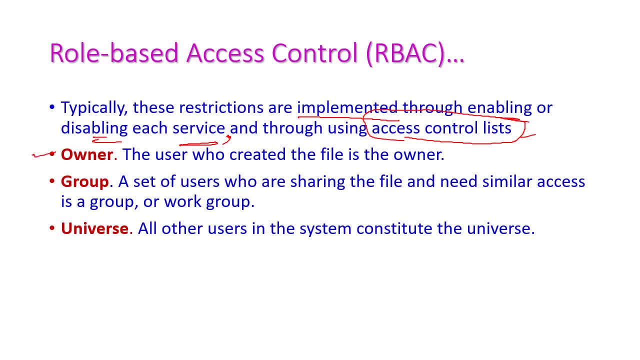 here we are having three different types of people. one, first one is owner. owner means who created the file. is the owner, who is the owner of the, the created data- okay, owner. and second one is group. group means a set of users who share the file. okay, and needs a similar access in a group or workgroup. that is, group means a people who are all working under.